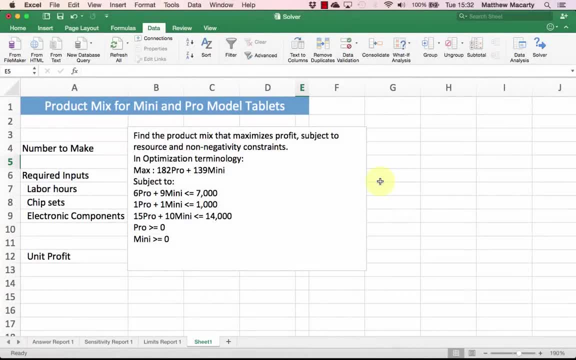 Okay, I'm going to go through a spreadsheet example of a linear programming optimization problem where we choose the optimal product mix for a relatively simple two-product mix, And I'm going to be using Excel Solver to do this. Okay, so optimization is a pretty powerful tool. It can be used in many situations where you're trying to find a scheduling solution, asset allocation, inventory control- And you know, in our situation we're using it to find a product mix. but it can be used in lots of different settings. 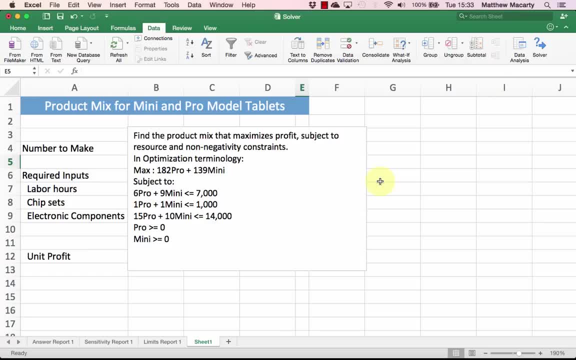 All right, and this is a linear problem, but you can be shown nonlinear And Solver can be used to solve those as well. All right. whether you're using a simple example, like I am, or a more complex example, these models tend to share many things in common. 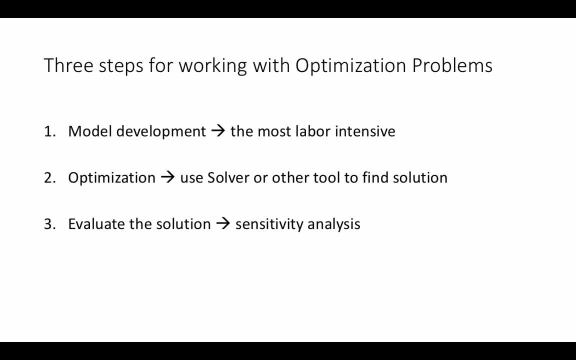 All right. so when you're working with optimization problems, you have basically three steps. The first step is the actual model development. All right, Solver is a really sophisticated. It's a really sophisticated tool, but it needs quite a bit of help to do its thing, And so we spend some time building the model. 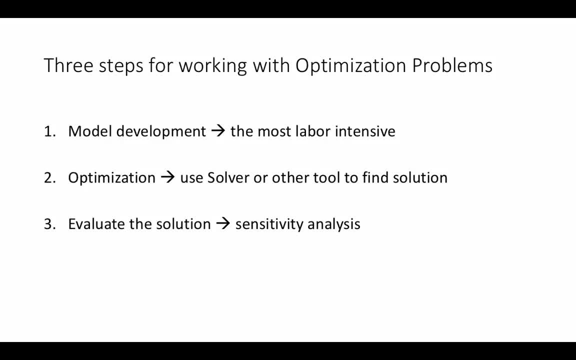 All right. the second step is actually using Solver or something like it to find an optimal solution. All right, and then, finally, you're going to evaluate the solution, because recognize that things in the real world may not work out the way they do in a model. 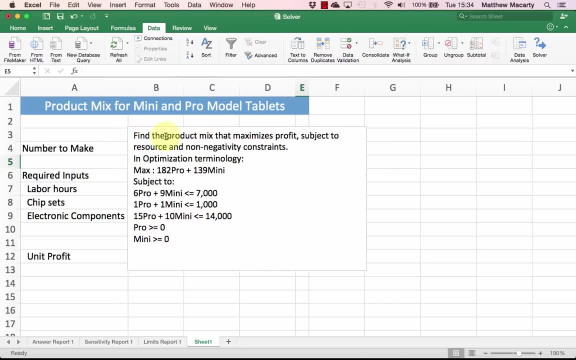 All right. so I've summarized the problem that we're going to be. We're going to be working on, We're going to be finding a profit mix that maximizes our profit And in this production run, we're limited to certain resources. 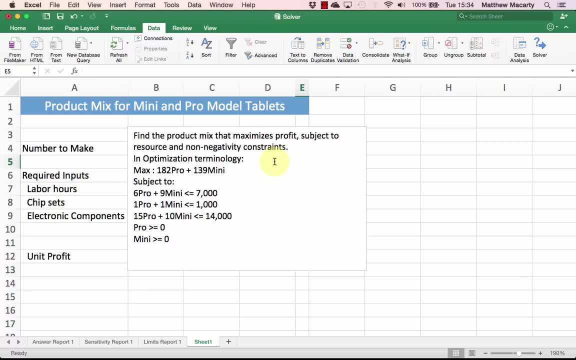 All right. and then, yeah, we're going to also tell Solver not to make any negative products, All right, so we're going to put in these non-negativity constraints. Okay, And when you work with a spreadsheet model, you're going to need basically four things in order to formulate something that Solver can actually solve. 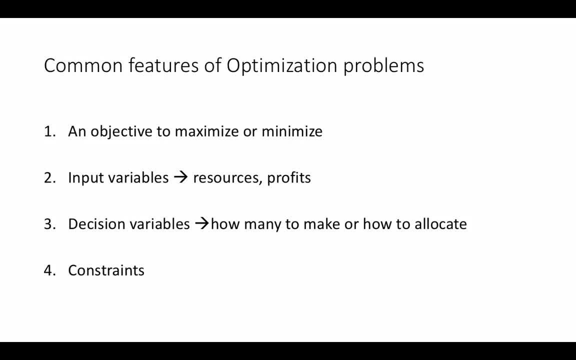 All right. so we're going to need an objective function, And the objective function is the thing that we're trying to maximize or, in some cases, minimize- All right. so in our case, we're going to try to maximize profit- All right, but you might be trying to minimize something like cost. 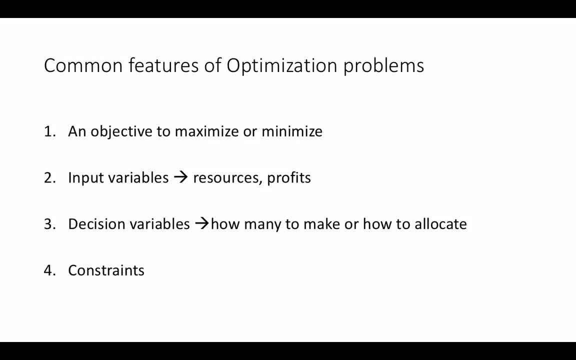 Or even risk, if you're talking about asset allocation, Okay, The second thing that these models are all going to need is input variables, So some kind of resources that are going to be used every time you make something, Or it could be the resources, dollars- that you're trying to allocate to some objective that you're trying to reach. 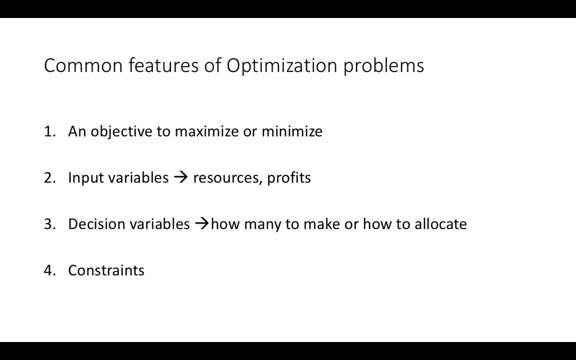 Okay, They all have decision variables, All right. The third thing is how many to make. In our case, that's what we're going to be working with: how many to make. But again, if you're talking about assets or something else, it may be allocating dollars. 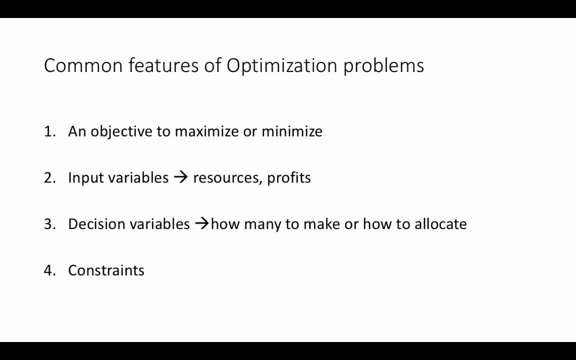 All right. And then they all have constraints. If you're missing one of these things, you won't be able to implement a model that Solver can solve. Okay, So I'm going to jump right into the model And I'll move this out of the way. 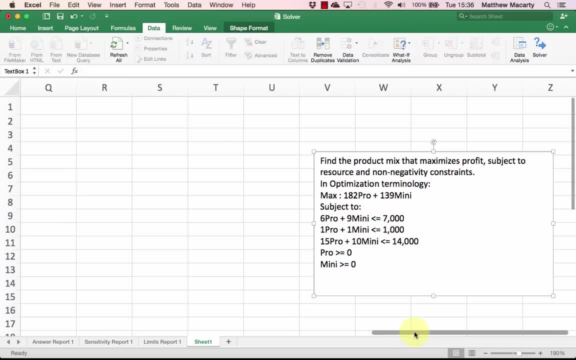 I've actually- Whoops, I'll move this out of the way. I'll move this out of the way. I'll move this out of the way. I've actually done a fair amount of the work to kind of facilitate this, All right. 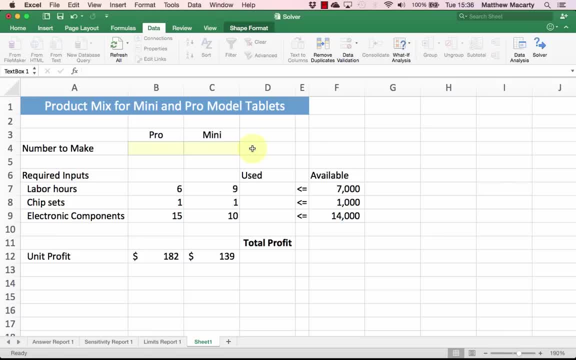 So I've sort of set up. you know, based on the inputs that we have, these are going to be our decision variables. I'll go ahead and put in some seed values there, All right. So basically I'm saying, okay, make one of each. 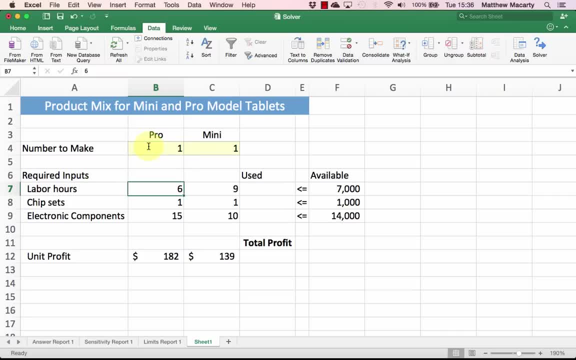 And then below I'm showing that for each unit we make, how many of each resource we use and then how much profit we make for each unit. Okay, Now I just need some formulas that sort of tally up when those input, those decision variables change. it sort of tallies up how much I've used. 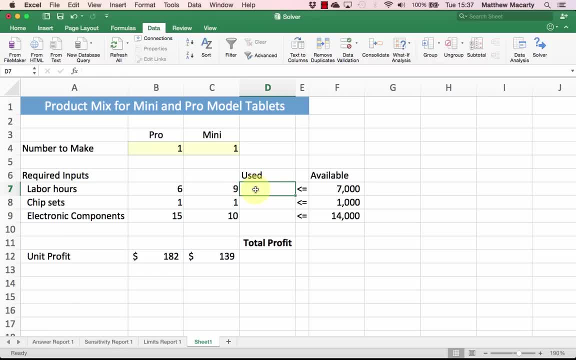 So I have something on the left-hand side of my constraint to compare to the right-hand side. Okay, So the formula that I'm going to use here: I'm basically going to take whatever's in B4, multiply that by 4.. 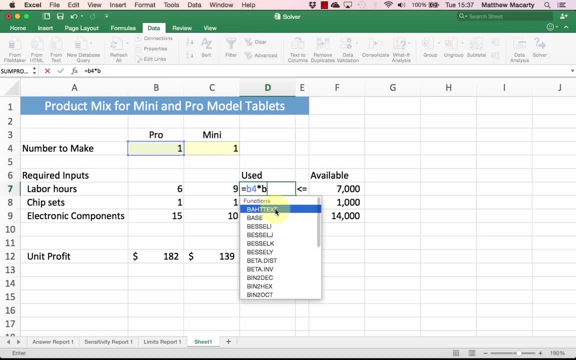 Okay, What's in B4, multiply it by what's in B7. And I'm going to add to that whatever's in C4 times C7. All right, So if we take a look at that, we can see that, okay, if you make one of each, you've used 15 labor hours in doing that. 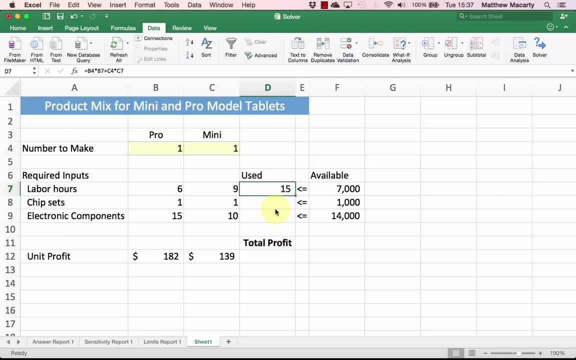 Okay, There is a shorthand formula for doing this, and it is the workhorse of these optimization models: It's the sum product function. Okay, So the sum product function does exactly what I just did, but it does it a little more compactly. 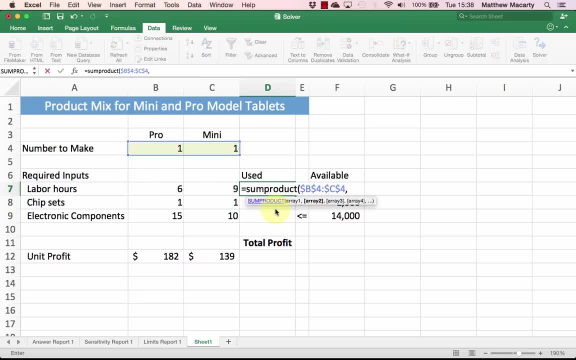 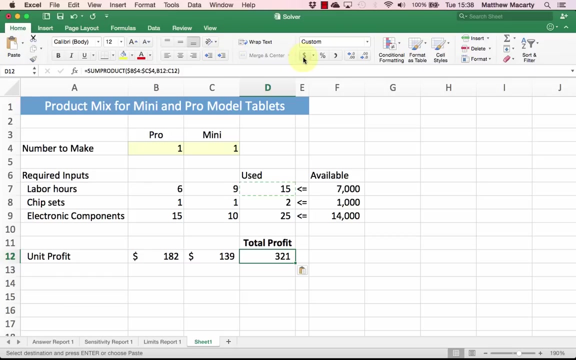 All right, And I'm using absolute reference here, so I can just copy the function down. Okay, Leave that one relative, and then I can just copy and paste All right And same formula down here. Okay, All right. So looking at our model, all right. if I just sort of go into this from a simplistic view, I might say: well, I make more if I make the pros, so why wouldn't I just sort of look at something simple like the amount of chips and use them all up and make pros? 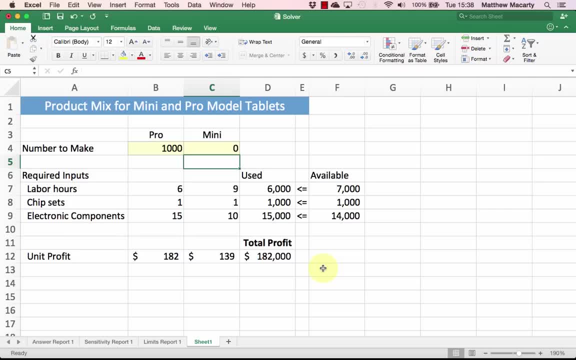 Okay, And so when I do that, sometimes that will work out. Okay, But when I do it in this situation, all right. yeah, I get a big profit here, but I've also used more components that are available, So this is not a feasible solution. 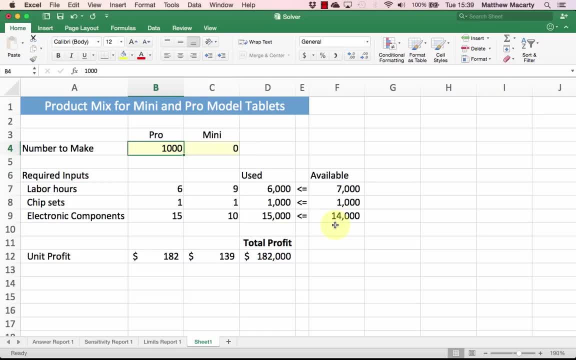 All right, And with a simple problem like this, right I can just start sort of by hand backing things out until I find a solution that works, All right. So just finding a solution that works doesn't sort of guarantee me that it's the optimal solution. 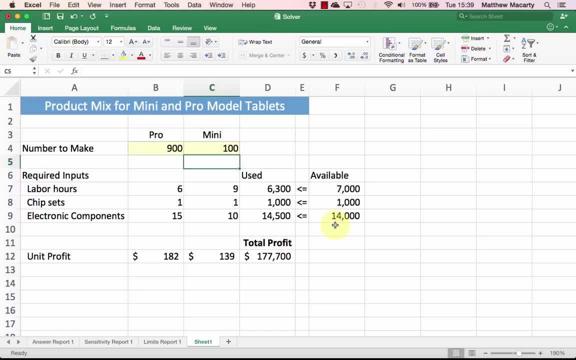 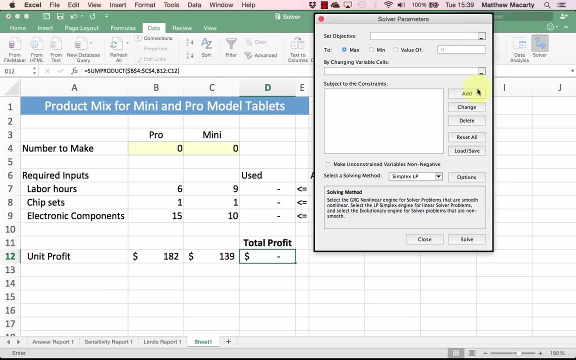 Okay. So in order to find that we're going to use Solver- Okay So I'm going to reset these to zero, I'm going to go to the data tab and I'm going to launch Solver. Okay, So Solver kind of corresponds to what I was saying earlier, that you need an objective. 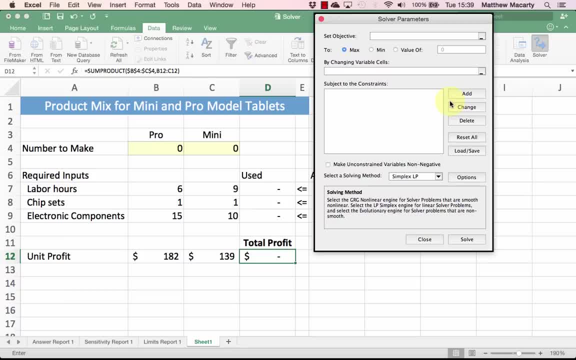 You need decision making, You need decision variables And you need the constraints. All right, So the objective here is our total profit. Okay, So I'll just point and click at that And you can see that. you know, by default it's maximizing that, but you also have the option to minimize or set it at a specific value. 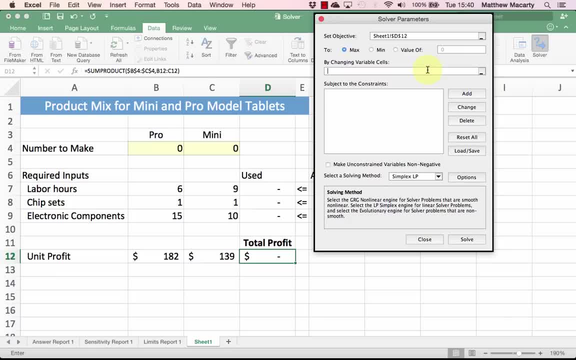 Okay, The next box is by changing variable cells. That's where the decision variables go, All right, So I'll point, click and drag on those. Okay, All right, And then it's going to be subject to some constraints. 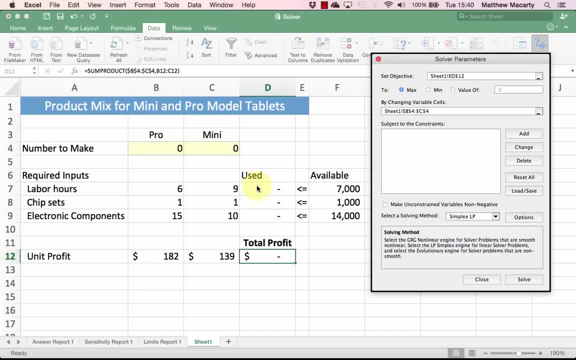 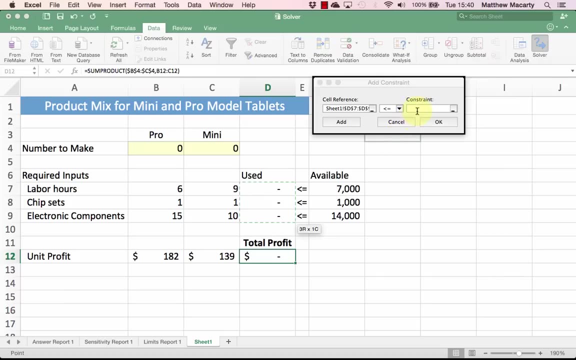 All right, There aren't any now, But basically we're going to say it's subject to all these values being less than or equal to these values. All right. So I'm going to click, add, All right, And again I'm going to point, click and drag. 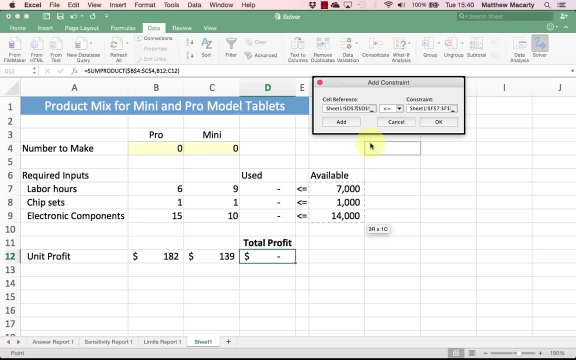 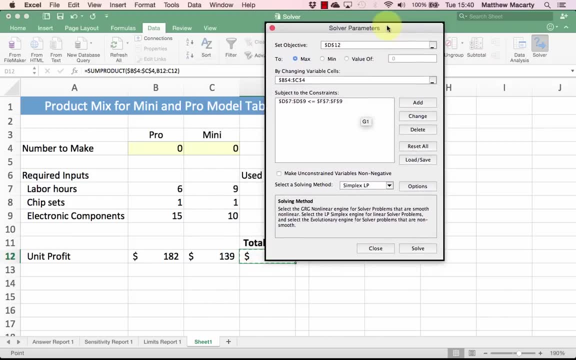 And then point, click and drag And click. okay, All right. So the other constraint that I mentioned: Solver actually knows that this is a pretty common one, All right, So it has a box down here that we can check. all right, to make the unconstrained variables non-negative. 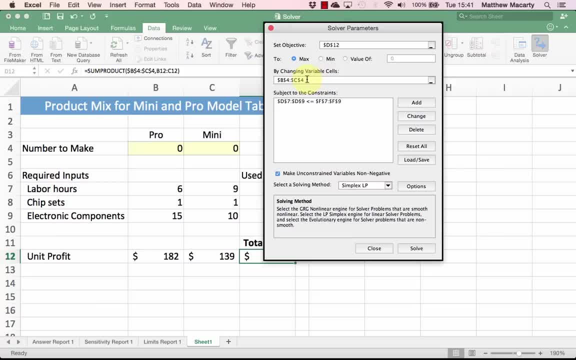 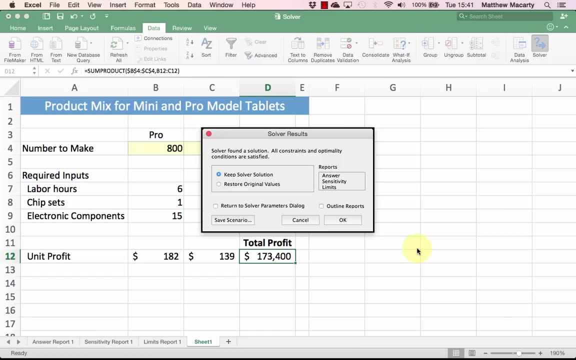 That's equivalent to saying: you know, these changing cells should not be negative. Okay, Once that's done, we can just click solve And, if I've set up the model correctly, in a few seconds it will give us a solution. 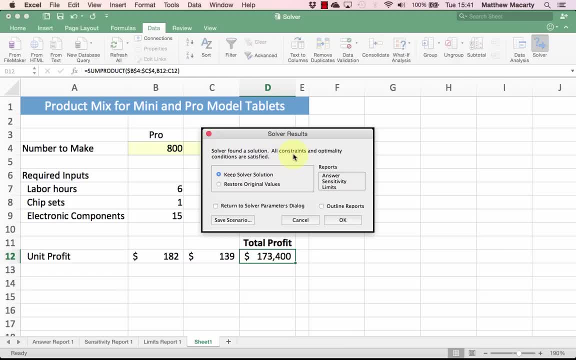 And this is the message we're looking for: Solver has found a solution, All right. Any other message that you see, it probably means you have to go back to the modeling step and try to fix something. All right. A lot of times what you'll see here is: Solver couldn't find a solution. 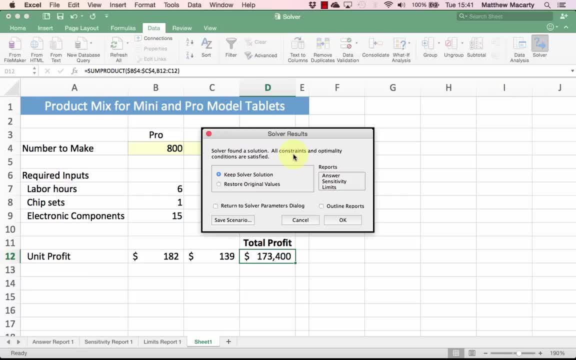 The problem is unbounded. All right, That really means that you have made one of your constraints- the inequality sort of point- in the wrong direction. Okay, So it does have a solution. All right Over here on the right of the box, you'll see. it has some reports that are available. 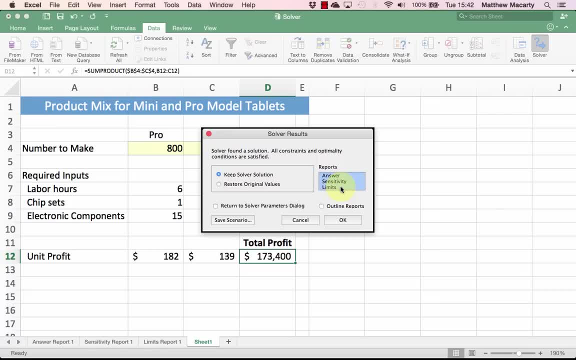 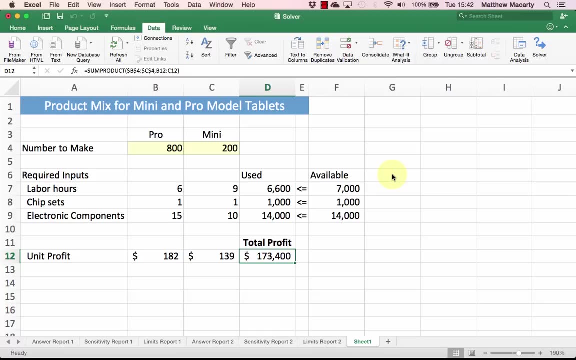 You actually have to click on each one of those to make them show up so you can evaluate the solution. I'll click, okay, And we can get a quick look at what it came up with for a solution And so we can see that. yeah, it doesn't tell us to make 1,000 pro. 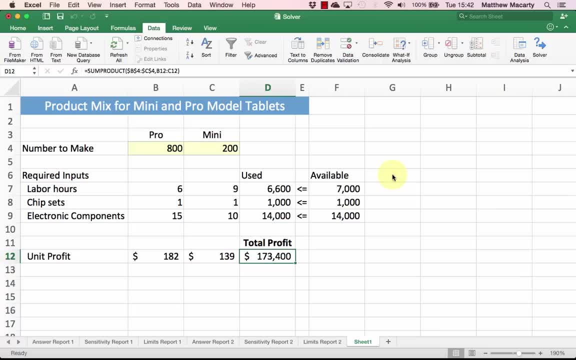 All right, And we know it wouldn't have told us that anyway. Based on the constraint, it couldn't go past 14,000.. All right, But it's told us to make 800 and 200 of the mini. All right. 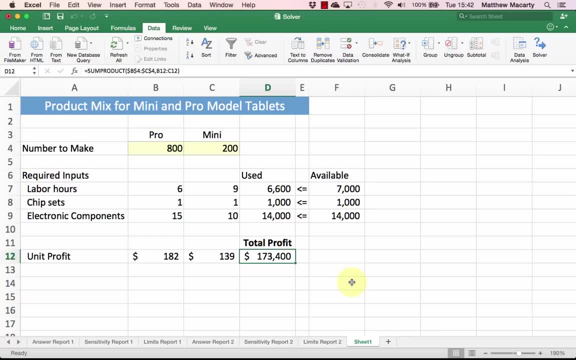 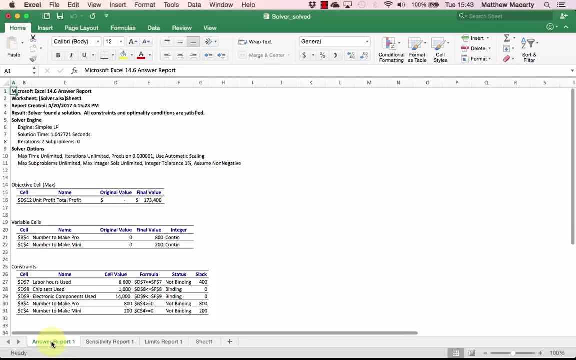 And then we get a profit of 173,400.. All right, So we're going to take a look at how sensitive that solution is to changes in any of the inputs. Okay, So I'm going to start on the first report, the answer report. 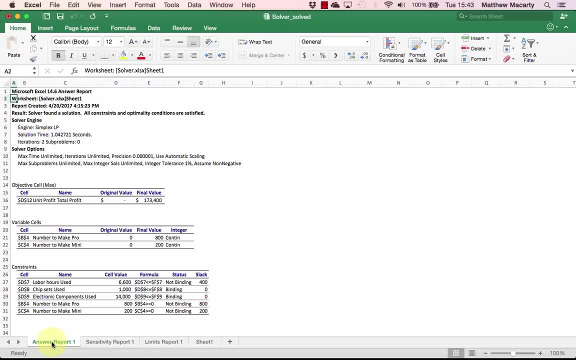 And it tells you some nice things like when you made the model and how many iterations it had to go through before it found a solution and then how long it took it to find that solution. All right, So it just tells you. you know, a lot of times you'll set up these models and you'll try to solve them by hand a little bit before you run Solver. for many reasons, 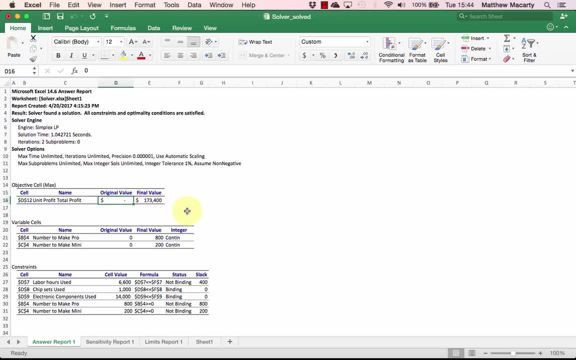 But you know we started at zero, so there's not a lot of information here. All right, We started at zero, We ended at 173,400.. Okay, It also says where the- you know- the decision variable started and where they ended. 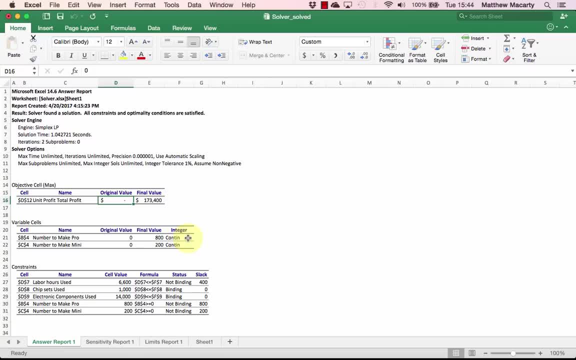 All right. The other thing here is that this problem is being solved as if everything in there is continuous. All right, Obviously we're not going to make partial tablets, We're not going to use partial resources, All right. But it's often easier to solve these as continuous variables. but then go ahead and interpret some of these reports as needed. 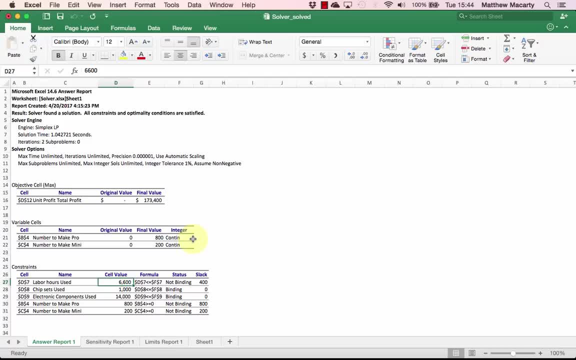 Okay, The other thing it really tells you down here is which variables you used- all of all right, and which you did not- All right. So the ones you used all of they are called binding All right. So there was no more left. 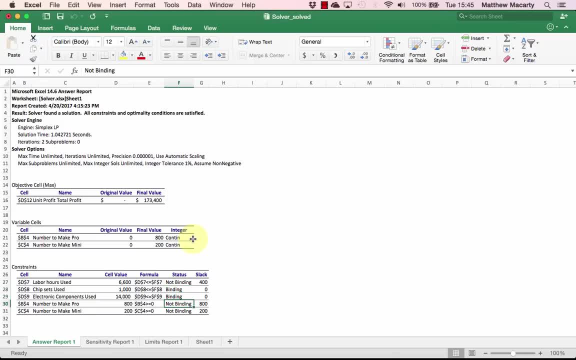 All right, There was labor hours left, All right. And basically it's saying that even if you hadn't put in the non-negativity constraint, that it would not have made negative or tried to solve this with negative values in either one of those cells. 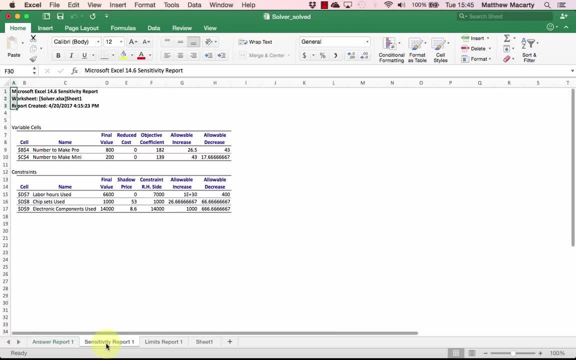 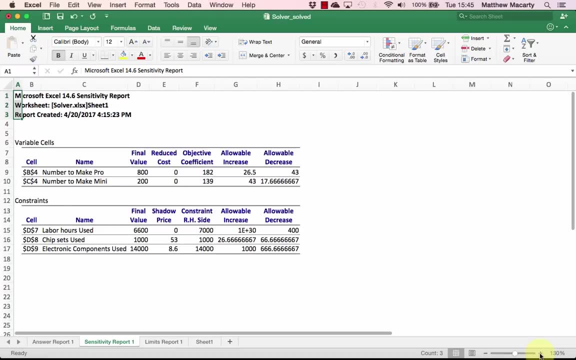 Okay, We're going to move on to the sensitivity report, and I'll zoom in a little bit so you can see it better, because this is the one that we probably spend the most time with. All right, It has two sections: It deals with the inputs, all right, the decision variables, and it deals then with the constraints. 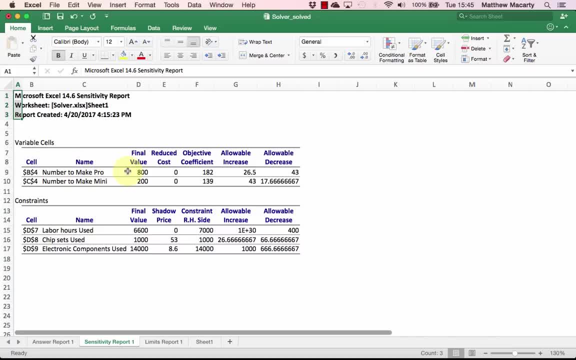 All right. So if we just look at the input variables, we can sort of see what the optimal solution is. No big mystery there. All right, It has this one column here: reduced cost. It shows that there's zero reduced cost. 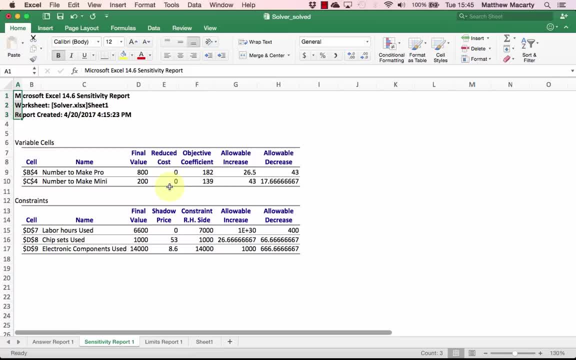 In a two-product mix, yeah, you usually don't see a reduced cost. All right, But if I added one product to this, if I had another model of tablet to make and allocate resources to, I might see a reduced cost and probably it would be negative, which would indicate that it would have a negative impact on the cost of the product. 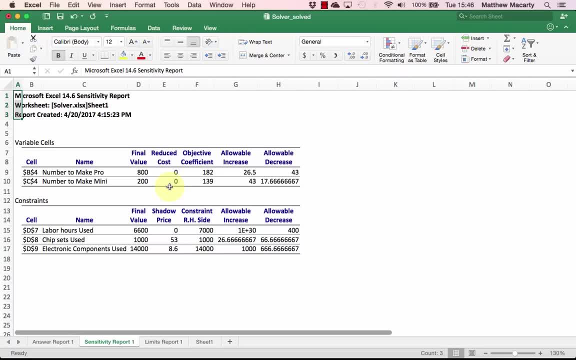 It would indicate that it would have a negative impact on the objective output, on the objective function. Okay, It shows you how much money you make- all right. or how much benefit you get from each unit you make, All right. And then it shows you here- this is the sensitivity part of it- 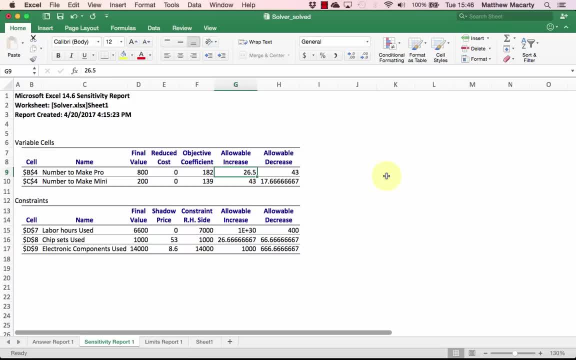 It shows you how much more you could, how much more the profit could be on the pro- all right- and how much less the profit would be on could be on the pro- Okay, Until you would get a different optimal solution. So in other words, I could increase, I could increase the amount of profit by up to 2650 or decrease it by up to $43, and I would still see the same product mix: 800, 200. 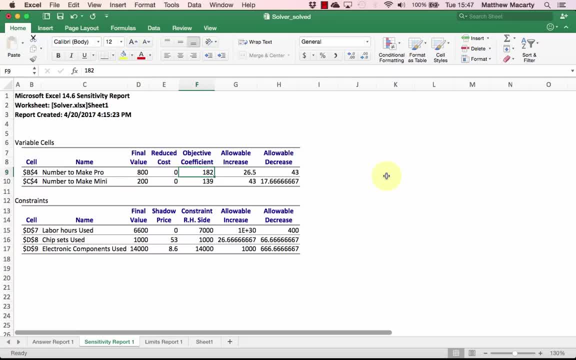 All right, If I go outside those limits then I'm going to start seeing a different product mix. All right, And we get similar numbers for the for the mini, Okay, So if I look at the constraint section, all right, it shows you again how much you used. all right, how much the optimal solution used. 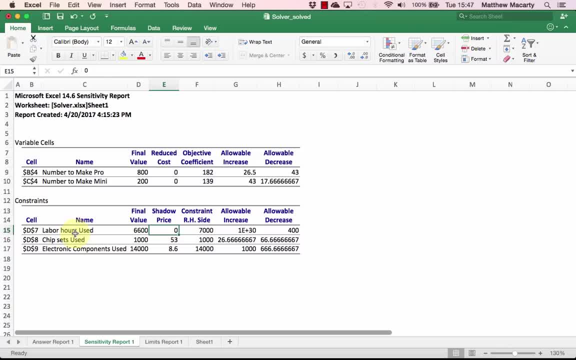 It has this other column called a shadow price. There isn't one for labor hours used, and that would be true of any constraint that was not binding, All right, So we we have some left over, and so there is no shadow price, All right. 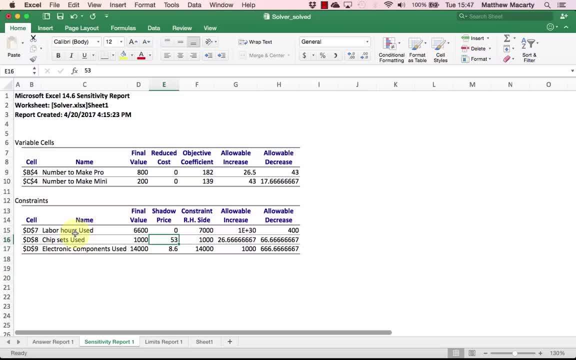 For the ones that we bumped up against those constraints. There's a shadow price in for chips It's 53. And what this is saying is if I had another chip and and if I had another chip, I'd also have to have more electronic components. 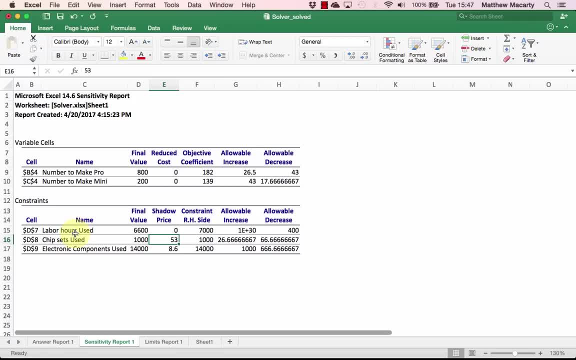 But if I just had another chip it would add $53 to that total profit, All right. And if I had another electronic component it would add $8.60 to that, to that, to that objective function, All right. So it basically shows you what a incremental increase in any of these resources, what that would do to the objective function. 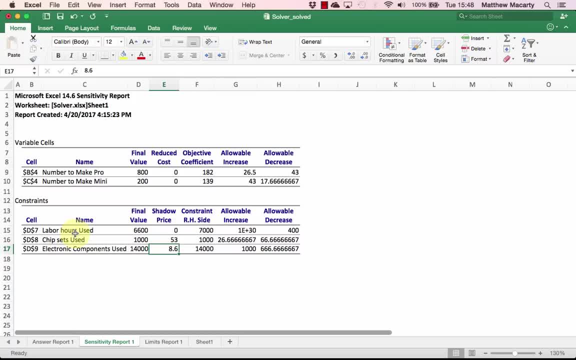 And it does that while holding everything else constant. Okay, All right. So no big mystery here. This, that's what the right hand side of the constraint looks like. All right, And then in this allowable increase, you know, since, no matter how much labor I added, it wouldn't change the objective function. 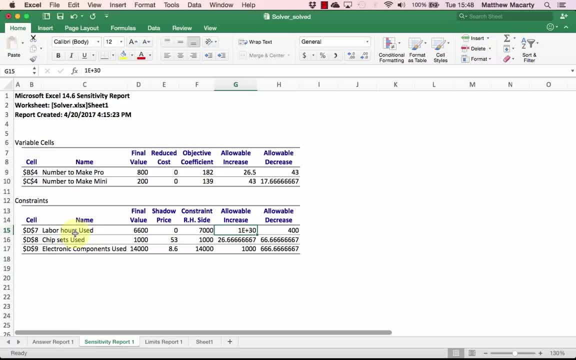 It's basically telling me I can increase that a lot. All right, That's sort of solvers answer for infinity. They're one times 10 to the 30th. Okay, It does show you that if I, if I have fewer, if I have 400 less hours, more than 400 less hours, then then I'd start seeing a shadow price over here.